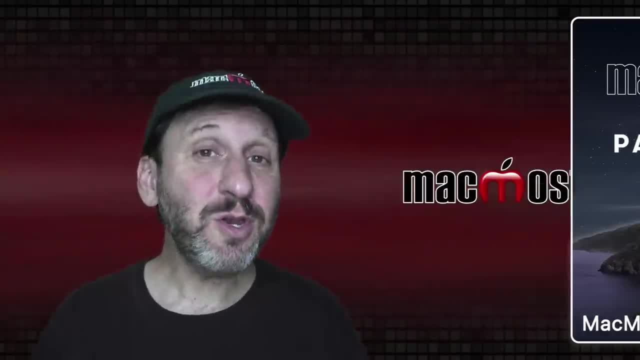 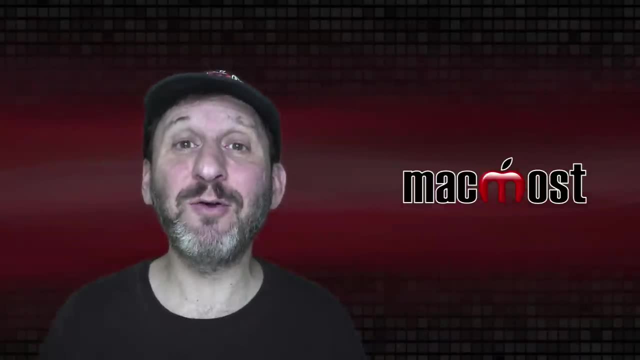 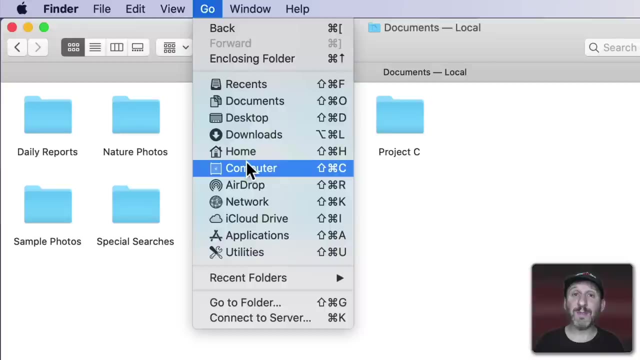 Join us and get exclusive content and course discounts, So you don't need to know why different folders and files are in different places on your Mac. But it can be useful to understand how your Mac works and get more out of it. So here I am with the Finder window and I'm going to go to the Computer level, So the top level. 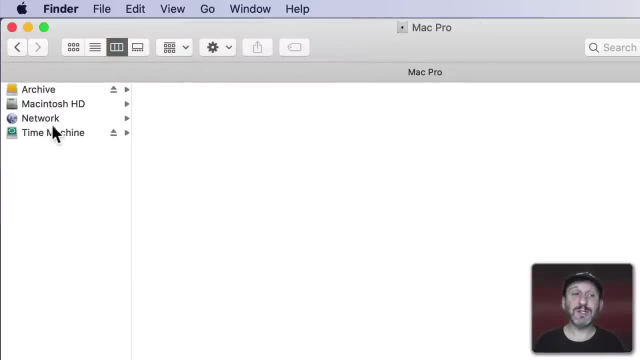 I'm also going to switch to Column View Now. here at the top level we'll see our main hard drive. You'll also see any other external drives. I've got two here and an item here to access Network things. But what we're interested in here is your Macintosh Hard Drive Now. 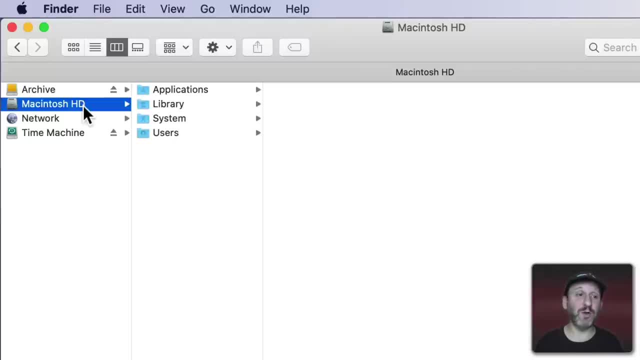 it may be called Macintosh HD, but it doesn't have to be. It could work, be called Mac HD, It could be called Gary's HD, It could be called anything, But for most of us it's going to be the default Macintosh HD. This is also referred to as the internal drive, or 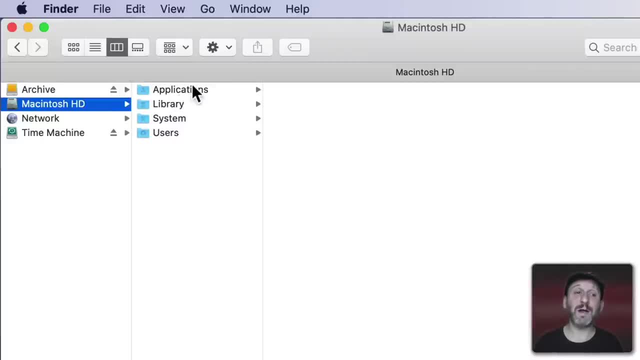 main drive of your Mac In macOS Catalina at the top level. we have four folders here. The first one that I want to point out is the System folder. This contains the macOS operating system. Catalina and beyond is also read only So you can actually go in here and 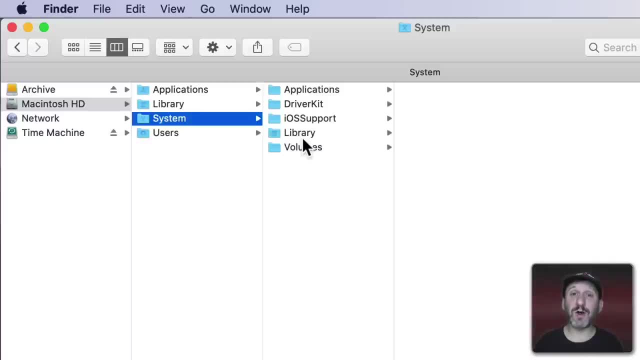 edit the files. You can look around and see what's there, But you can't do anything to alter them, at least not easily. This is a good thing because it protects your system against malware, because even if you install a piece of malware, it can't write to the system, So it can't change how. 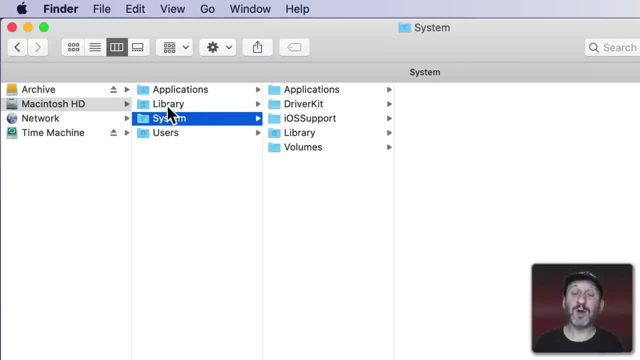 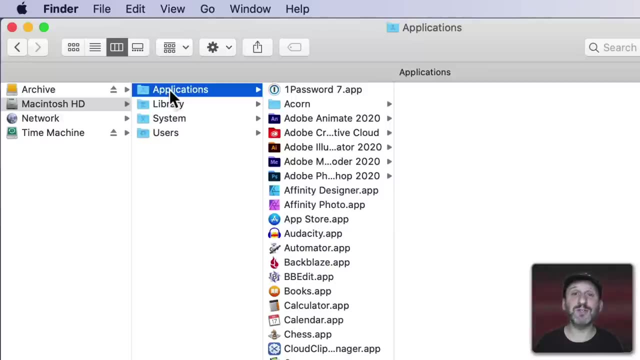 macOS works. You also have three other folders here. One is called the Applications folder. This contains apps, Things like Pages, Numbers, Keynote, TextEdit, Mail, Safari. Any app that you install on your Mac is probably going to end up here. 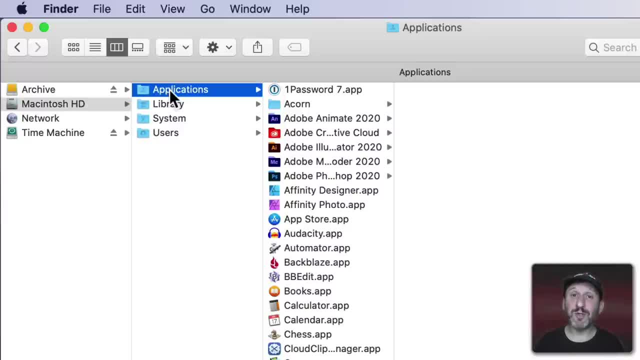 The reason this is at the system level is that if you have multiple user accounts on your Mac- say for you and your spouse- you can share the same apps. You don't have to install Pages and your spouse install Pages as well. You install it once on the computer and both user accounts can access Pages. 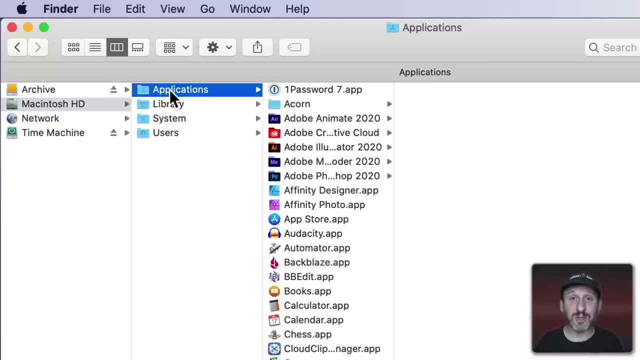 So when you install a new app, say in the Mac App Store or using a third party app installer, it's going to end up here at the system level or main level in the Applications folder. Now you also have a folder here called Library. 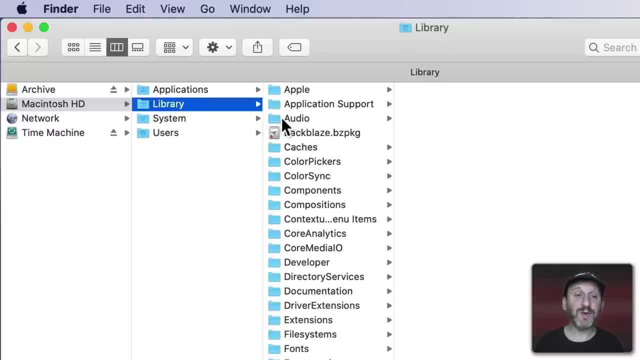 This will contain support files for different apps. So for instance here, if I look in the Audio folder here, I'll see various things that are used by GarageBand- maybe Logic Pro, if you have that. maybe other music and audio recording apps as well. The idea here is the applications. 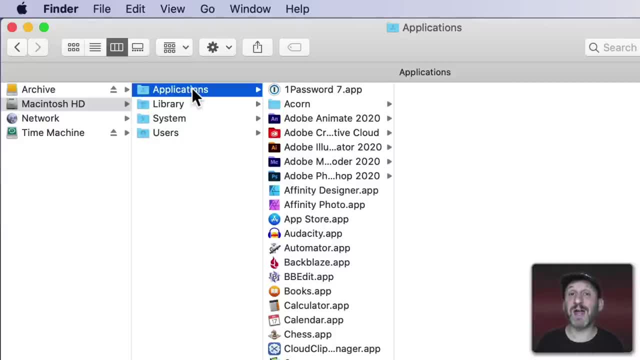 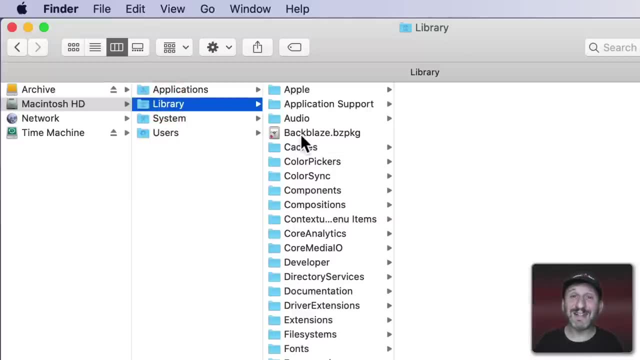 themselves are exactly the applications. If you have an application and I have an application, we have the same file here, But in the Library we may have different things. I may have installed extra plugins, content, themes, all sorts of things for different apps. 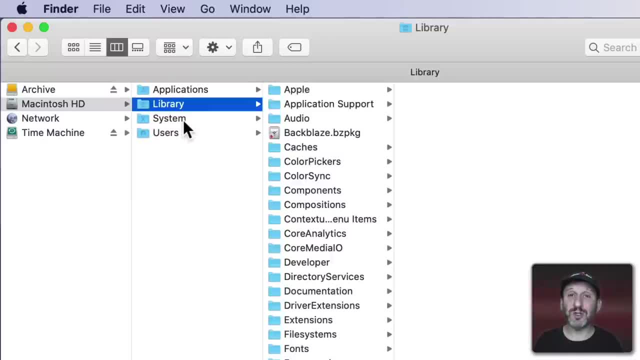 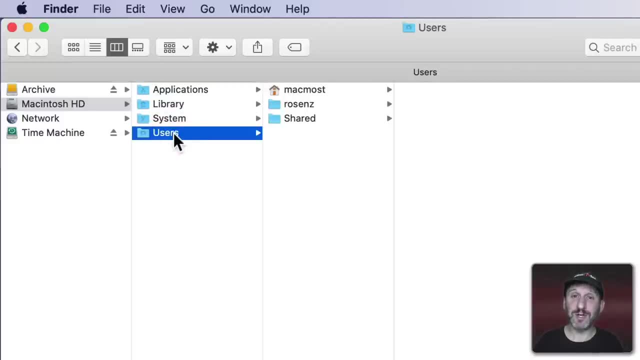 They would go into the System Library folder. Now, in general, you never need to look at or mess around with the System Library or Applications folder, But the Users folder. that's where your stuff is going to be Now. in the Users folder there's going to be a separate folder for every. 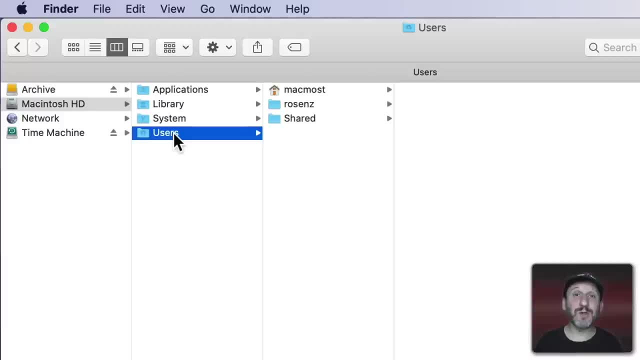 user on your Mac. For most of us, only one person uses the Mac, so we only have one user account. But you could have a situation where you have multiple people using the same Mac and they should each have their own user account. Each user account could have its own iCloud. 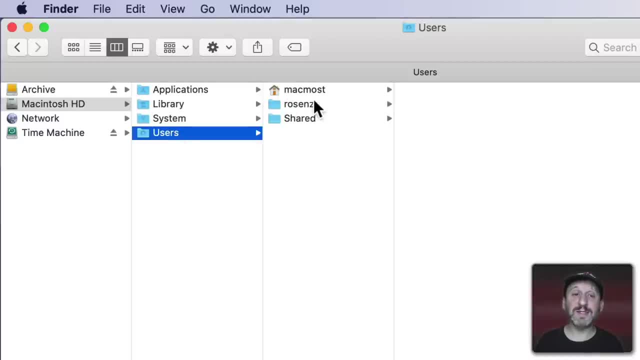 account. It could have its own files, settings and other things. In this case, I have two user accounts here. One is my main user account that I use for creating apps, maintaining websites, doing things like that. Another one, the one I'm currently using. 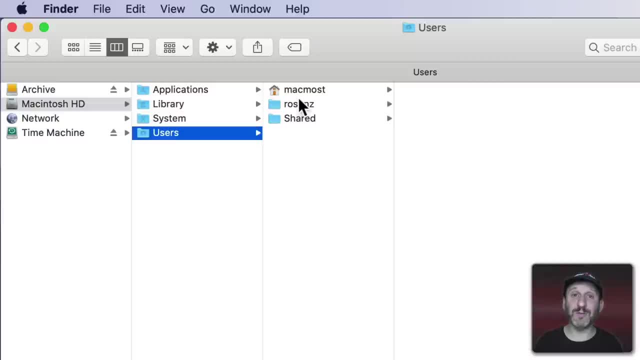 and you can see it has a little house icon to indicate it's the user account I'm currently using. that's this one and I use it to make tutorials. You also may find a Shared folder in here. That's a way for you to share files easily between user accounts. So if you go with 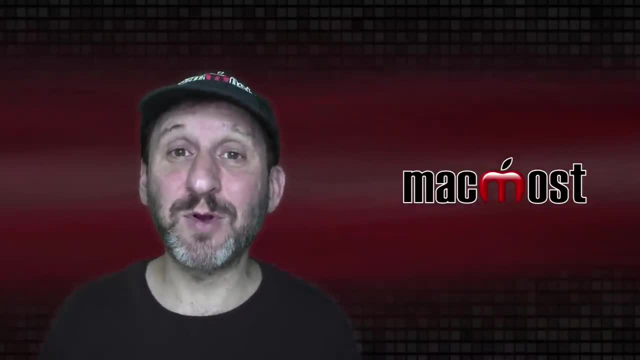 an apartment metaphor. you could think of each user account as a separate apartment, Only the person with the key, their password, and you can't get into somebody else's apartment. The system and library are like the building itself: It's the structure, things like the water pipes. 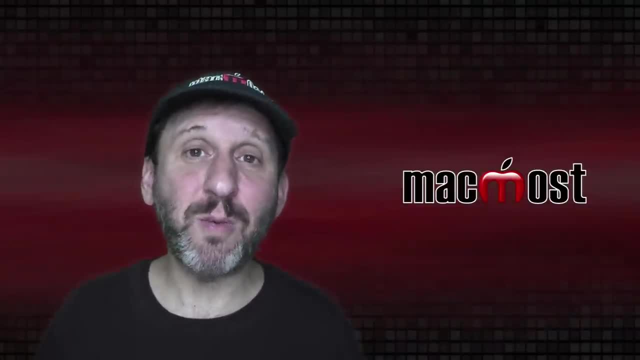 the electricity and things that everybody accesses, Like maybe the entryway and the workout room and the hallways and the stairs and the elevator. The Shared folder is like a common room that anybody with an apartment can access, but most people probably don't use it. Now, when 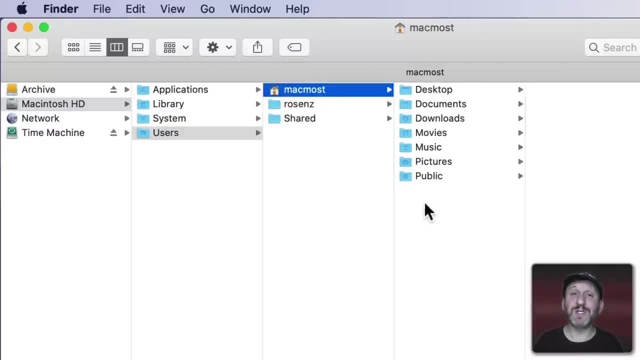 we go into a User folder. we're going to see some common folders in here, So chances are you have some common folders, Maybe more. Most notably, there's your Desktop and Documents folder. These are the two places where you can put all of your files. So when you create files using 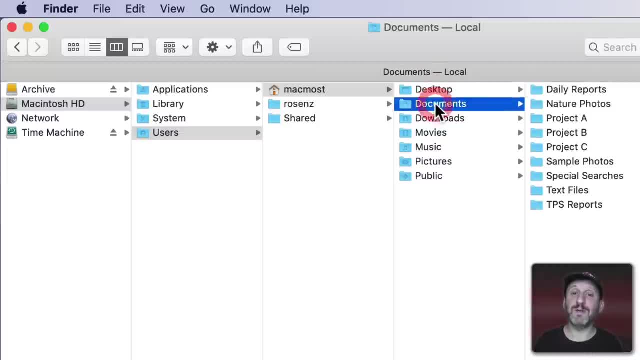 different apps or download things. you can put them in the Desktop or Documents folder. Best practice is to store as much as you can in your Documents folder and create folders inside of here to organize things. Some people may only have a handful of files and just have them in. 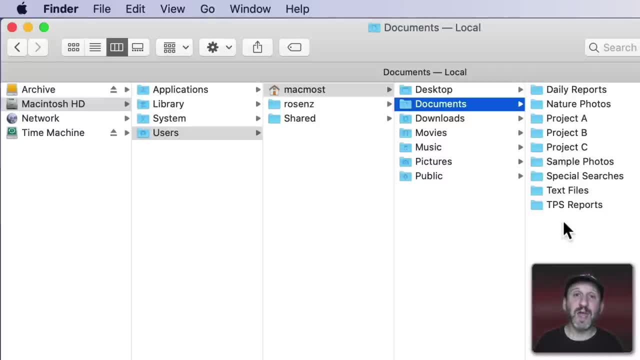 their Documents folder. Other people may have hundreds or thousands of files and may want to organize them into folders and subfolders, So that's a great way to organize things, And everybody's Documents folder is going to look a little different. You can also use the Desktop folder in a similar way, except that the Desktop folder has a special 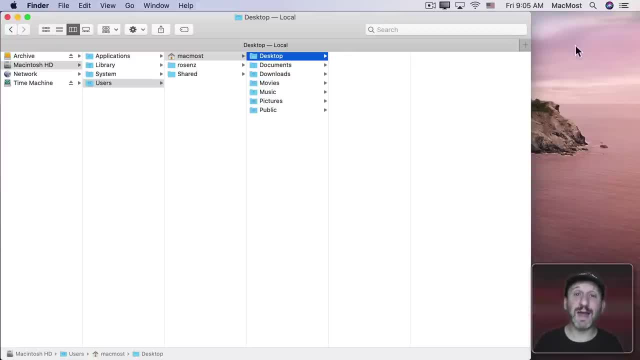 property that anything that's in here is also going to appear on the Desktop. here. It's just two ways of viewing the same files. So if you put too much stuff in your Desktop folder, it's going to clutter up the Desktop, Which is why it's a good idea to put a majority of your stuff in here. 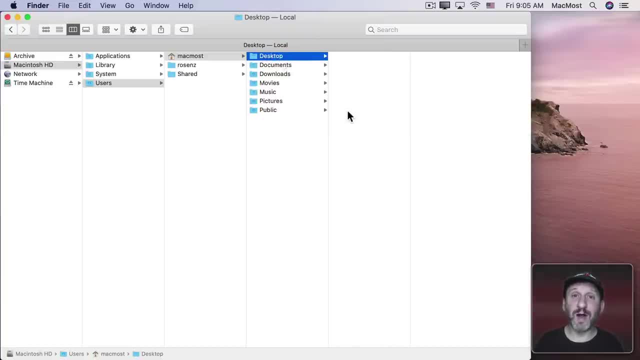 and keep your Desktop clean, or maybe just one or two files that are there temporarily, or things you access all the time. So that's a great way to organize things. So that's a great way to organize things. Now, the rest of these folders are here for special reasons and you're probably going to 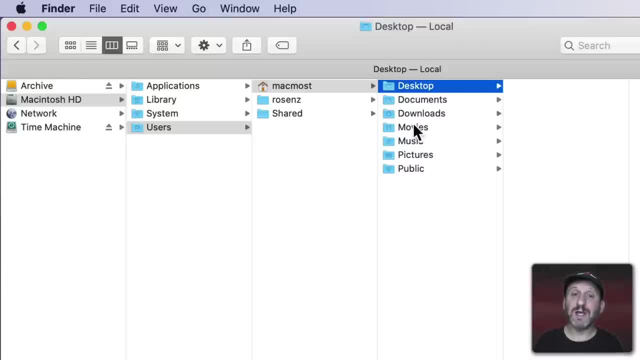 find similar files in here to what others have. For instance, in your Movies folder you're probably going to find things like your iMovie Library folder. if you use iMovie, You may also find other apps that use video to store things here, Like, for instance, I have the Screenflow. 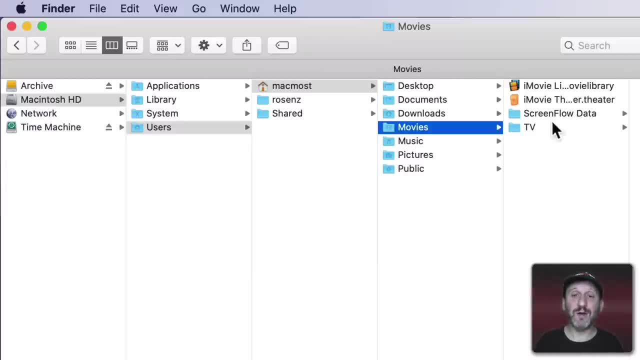 app that records these tutorials and puts a folder here as well. The TV app also uses a folder here. The same thing is true for Music and Pictures. In the Music folder I find another music folder for the music app storing my music library. But I also find a folder for Garage. 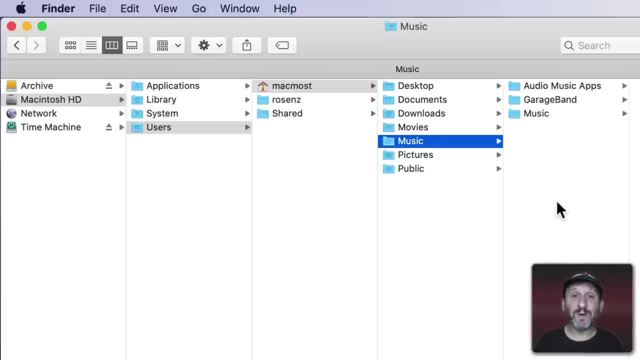 Band and some other apps as well. You may have different folders in here depending upon which music or audio apps you use. In the Pictures folder I have just my Photos Library, But if you have other apps that use the Pictures folder, they may store their libraries or have folders. 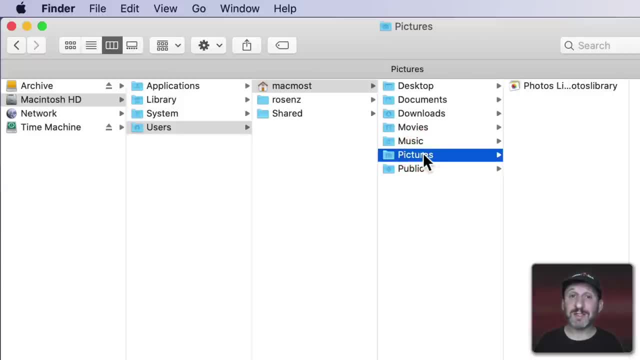 in here as well. Now, Movies, Music and Pictures folders are completely accessible by you. You can create your own folders in here if you want or never use them, For instance, in the Pictures folder. if you have a large clipart collection you purchased that you use for work, you may want to. 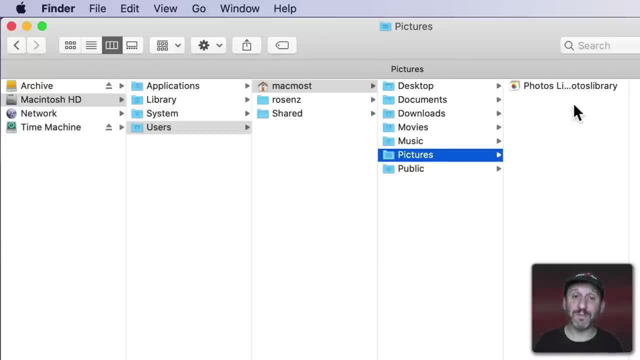 put that in here. It may make sense to store them in the Pictures folder In Movies. if, say, you've downloaded a bunch of videos or you've created a bunch of videos and you want a good place to put them and you don't want to put them in your Documents folder, you could put them here. It's. 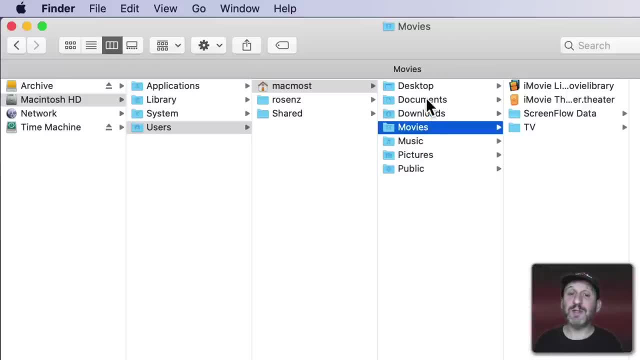 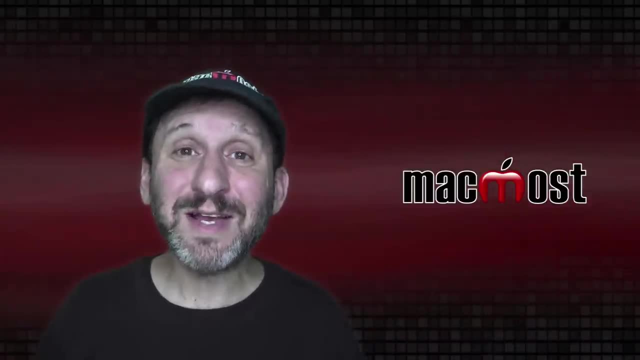 up to you. You could put them in these folders or you could put them in your Documents folder. If you think of this like an apartment, your Movies folder could be, say, like your kitchen, and Videos could be like food. It kind of makes sense to put the food in the kitchen, but you don't. 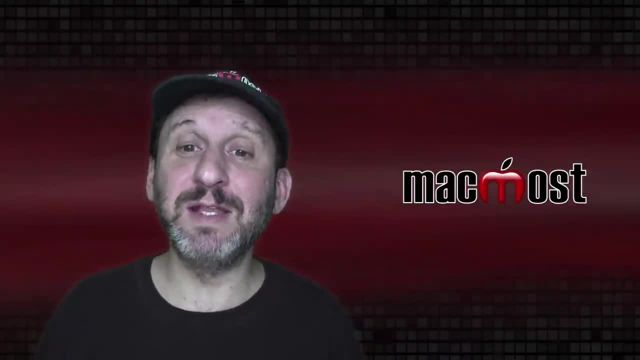 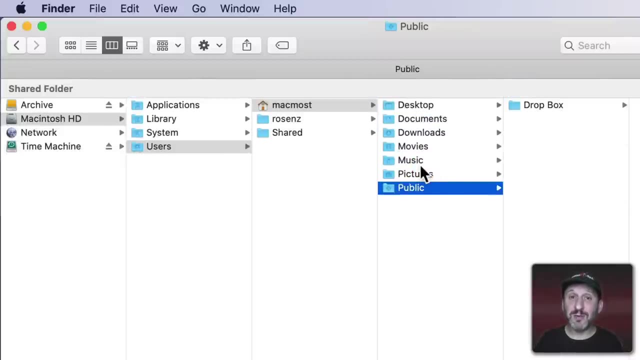 want to, But nobody is going to stop you if you want to put, say, a bag of chips in the living room instead of in the kitchen. Now you may also see a Public folder. A Public folder is a folder that not only you can access, but other users on your Mac can access as well, So most of us may. 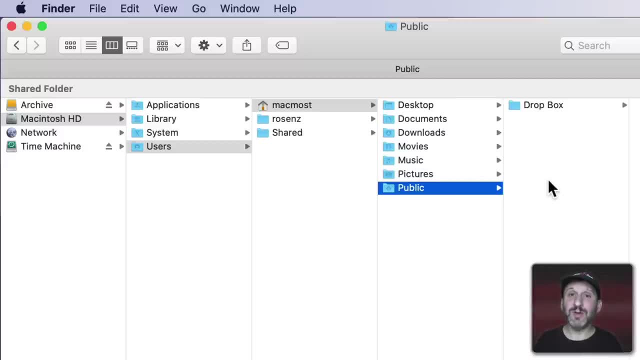 not use this, but if you do put something in here, a second user could actually see that file In the Dropbox folder in there. somebody can actually put something in that file, So only people on your computer that can access these. There's also the Downloads folder. The Downloads folder is a. 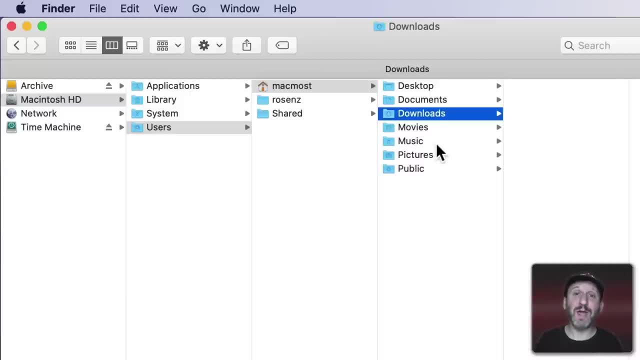 default place for apps like Safari and other browsers and Mail to save files. Other apps that you get that download files may also use the Downloads folder as a default location. There's nothing to prevent you from downloading a file and saving it to your Documents folder, for instance. 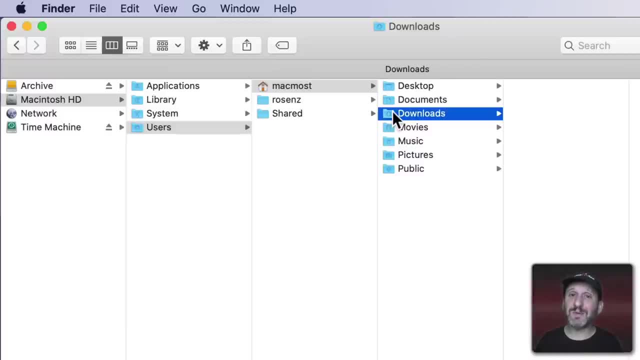 The Downloads folder is just a convenient location for those things to go. A lot of times we download something and only need it temporarily, Like an installer for an app. You run the installer, it installs the app and now you want to get rid of the installer. 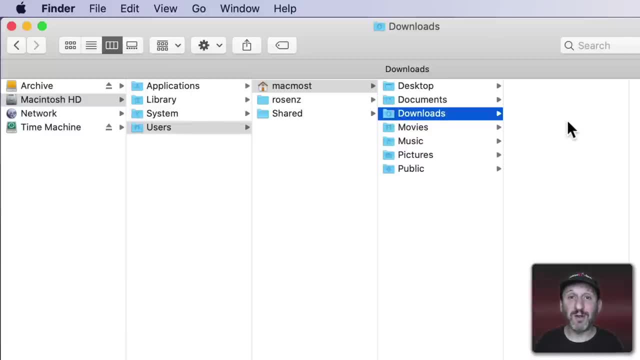 So it's just sitting there in your Downloads folder, A convenient place for you to then go to find it and delete it. Other times you may download, say, an image, and just want to view it, but we don't necessarily want to store it anywhere It goes. 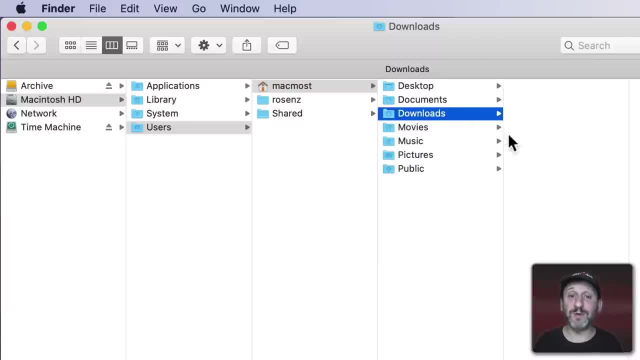 to the Downloads folder temporarily. We can then move it to our Documents folder, move it to the Pictures folder or throw it away. Now another location for your files would be iCloud Drive. If you're using iCloud Drive, you can do Go and then choose iCloud Drive. This looks like a. 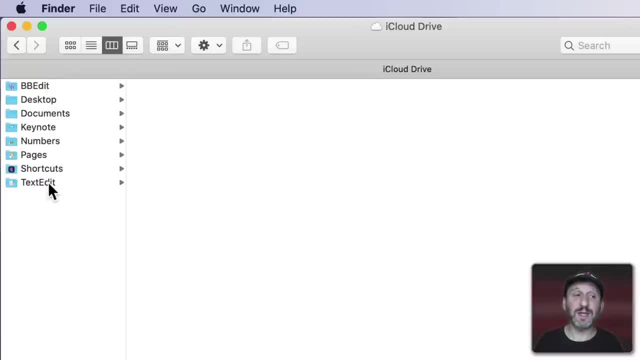 completely separate location where you have various folders for things. So for instance, that create folders for convenient storage for things like a Pages or Numbers folder. You may also see a Desktop and Documents folder in here. In fact, if you go to System Preferences. 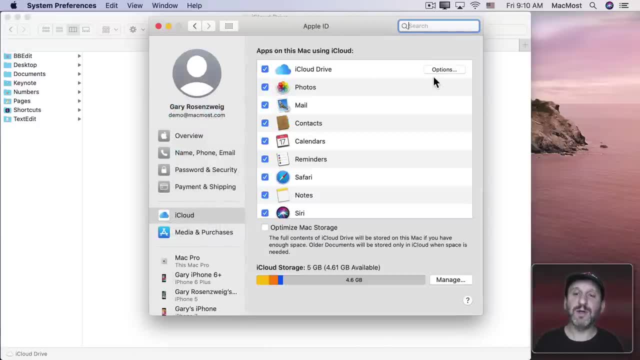 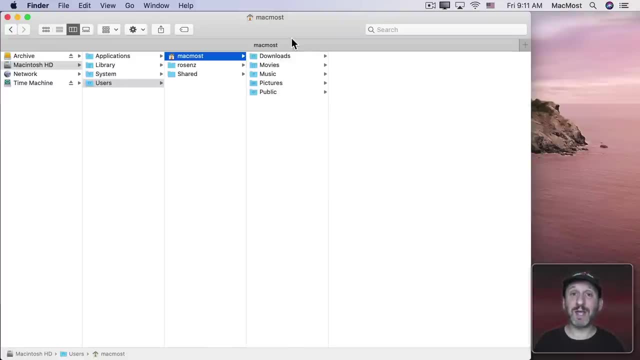 and then your Apple ID and then iCloud, iCloud Drive Options, and turn on Desktop and Documents folders. now you'll find in your Home folder that Desktop and Documents folders aren't there anymore. They've now moved to iCloud. You still use them for the same things. If I choose, Go and 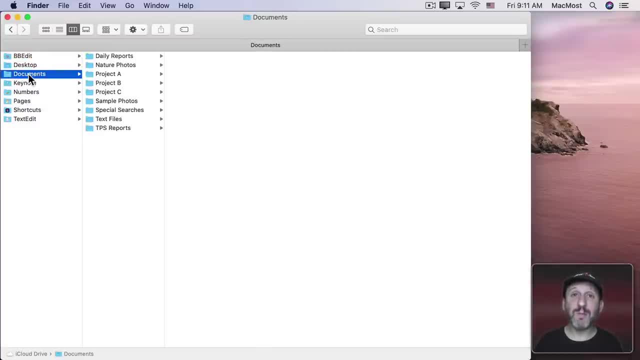 then hold the Option key down, Library appears and I can select it. Now you can see it was there, It was just hidden. The Library folder in your Home folder is the same folder that I used to use, So I can see here my Desktop folder, my Documents folder. they work the same way. They're just. 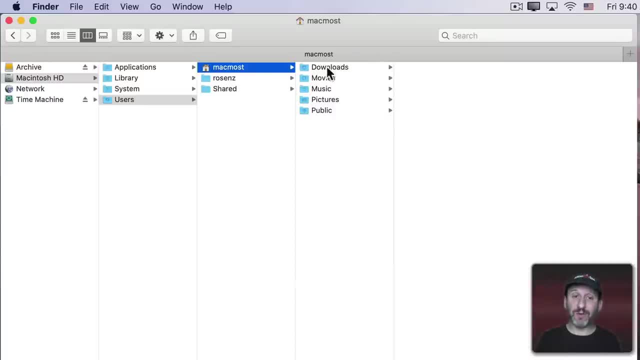 located in iCloud now, which means that I'll be able to see the same Desktop and Documents folders on all of my devices. Now, one folder I haven't mentioned is your Home Library folder. You don't see it here. In your Home folder you don't see a Library folder. But if you choose, Go and then hold. 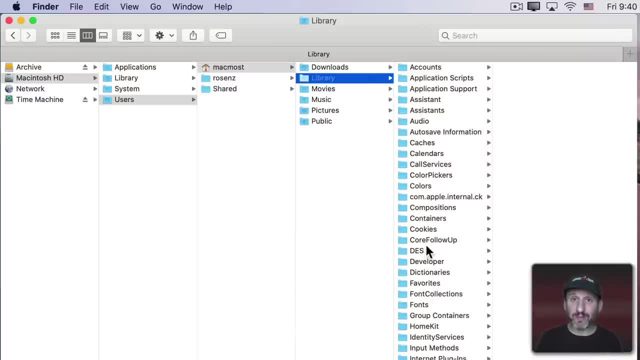 Home folder. it's like the System Library folder, except it contains support files for applications that are specific to you as a user. So for instance, in here you'll see Preferences. These are little preference files for your applications. So for instance, if you've gone, 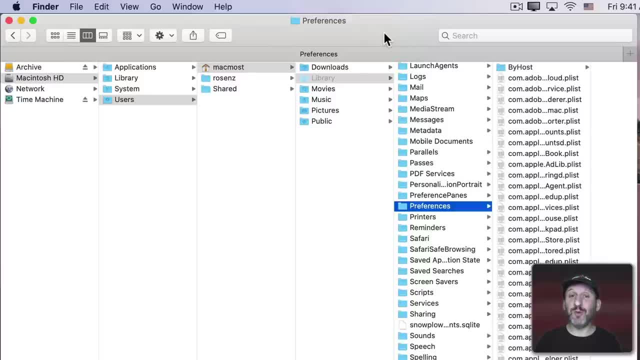 into an app and changed one of the preferences there- that's for you and your user account- Somebody else with a user account on your Mac- they would have their own set of preferences and they would all be stored in their own Library folder, in their Home folder. 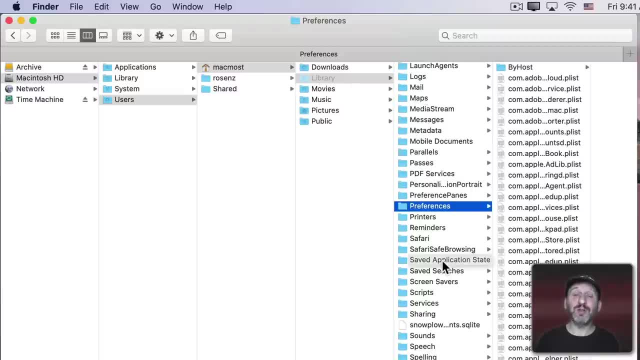 And all the other things in here also pertain to you as a user. So storage for Settings, storage for Data for different apps- they're all here in the Library folder. The reason it's hidden is because there's really nothing in here for you to control directly. The apps themselves are in. 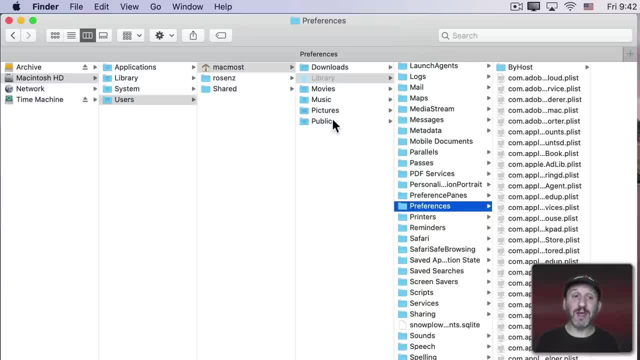 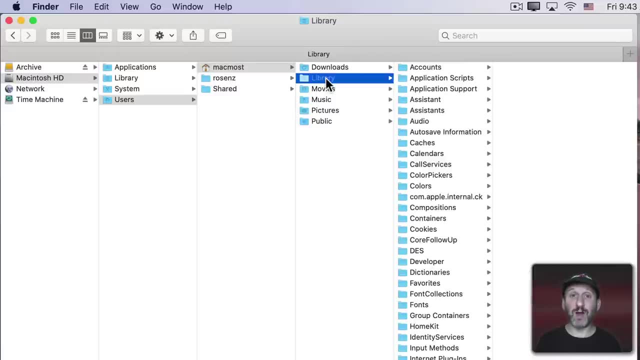 charge of accessing and modifying all the things in the Library folder, and there's really not much for a regular user to do in here. That's why it's hidden. One last thing I want to point out is that if you're using iCloud Drive and you have your Desktop and Documents folders stored there- Movies,